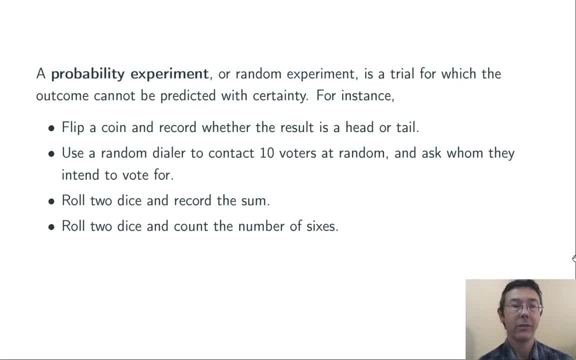 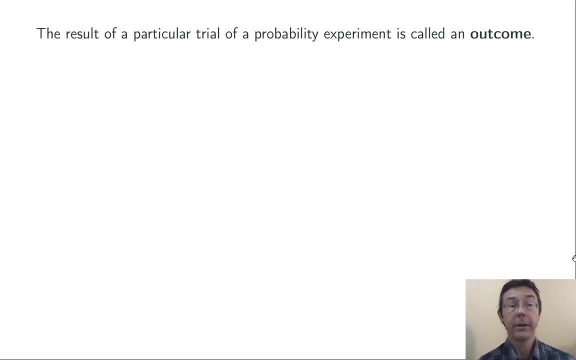 the sum, Roll two dice and count the number of sixes. By the way, notice, in these last two cases we're doing the same action, but the data that we're recording is slightly different. So we have different probability experiments. A little bit more vocabulary. 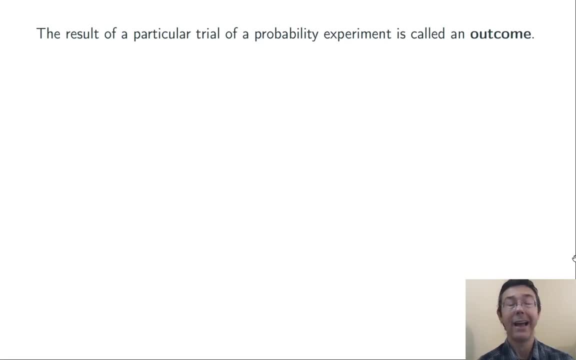 The result of a particular trial of a probability experiment is called the outcome. The collection of all possible outcomes of a probability experiment is called the sample space or outcome space, usually denoted with a capital S, and a subset of the sample space is called an event. I think this all makes more sense when we 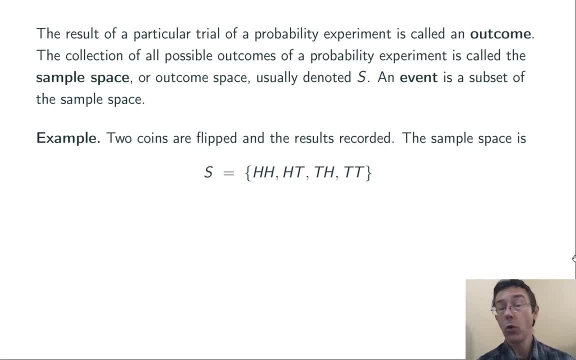 do an example. so here we go. let's flip two coins and just record the results. the sample space consists of four outcomes: heads, heads, heads, tails, tails, heads and tails, tails. if we let e be the event both flips are the same, then we have two outcomes in that event: heads, heads, tails, tails. this is a subset of 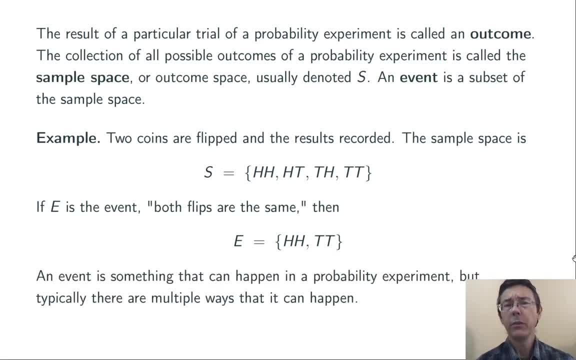 the sample space. roughly speaking, an event is something that can happen when you run the probability experiment, but there may be multiple different ways that it can happen, as in this last example, the event- both flips are the same- can happen two different ways. if you have an event that can only happen one way, in other words, the event 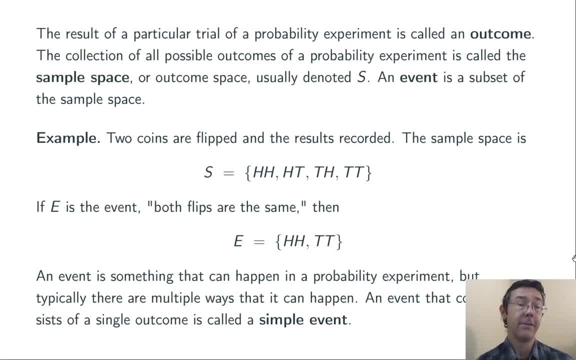 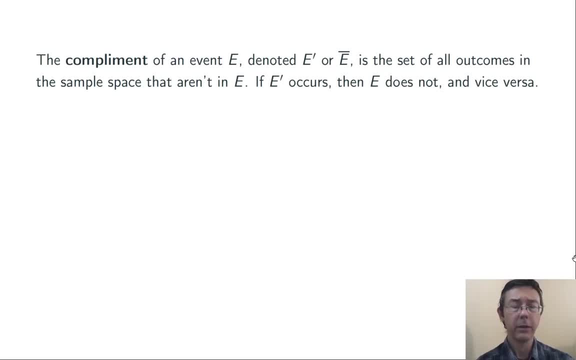 consists of a single outcome. we call that a simple event, the complement of an event, e usually denoted e prime, sometimes e with the bar over it- is the set of all outcomes in the sample space that aren't in e. so if e occurs then e prime does not occur, and if e prime occurs then e does not. for instance, 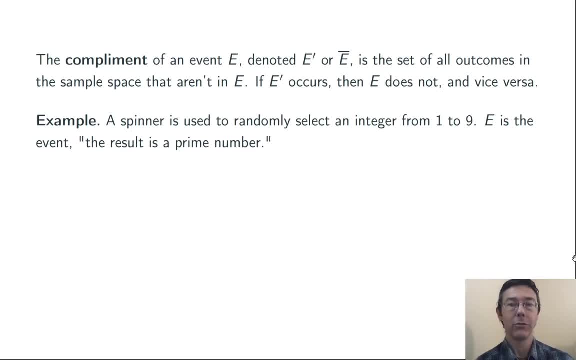 suppose an event is an event that has multiple outcomes in it. so we have an, we use a spinner to randomly select an integer from one to nine and let e be the event. the result is a prime number. here's the sample space. it's just the integers from one to nine, and here's 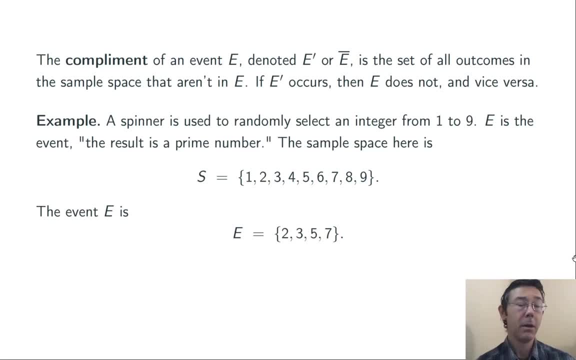 the event e. written as a set it's all the prime numbers that are less than ten: two, three, five and seven. so the complement of e, e prime, is going to be the event that e does not occur, so written as a set it's going to be all the numbers less than 10 that are not prime 1, 4, 6, 8 and 9.. 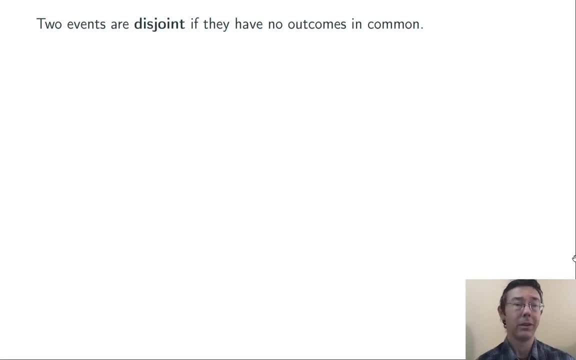 two events are disjoint if they don't have any outcomes in common. to say it differently, if they can't both occur. for example, flip four coins and record the results and let e be the event. the first two flips are heads and f. there are at least three tails. 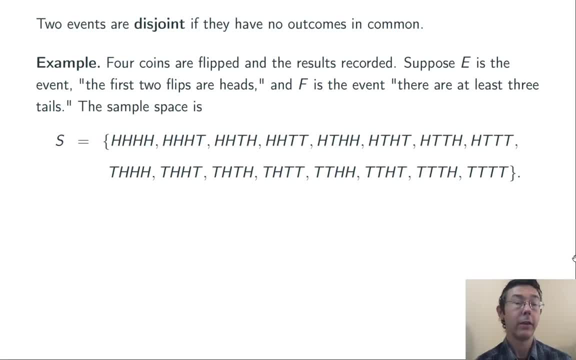 so the probability experiment can sit. has a sample space that consists of 16 possible outcomes. things like heads, heads, heads, heads and heads, heads, heads. tails e and f can be written as follows: e- the event- the first two flips are heads- has four outcomes. in that event, things like heads. 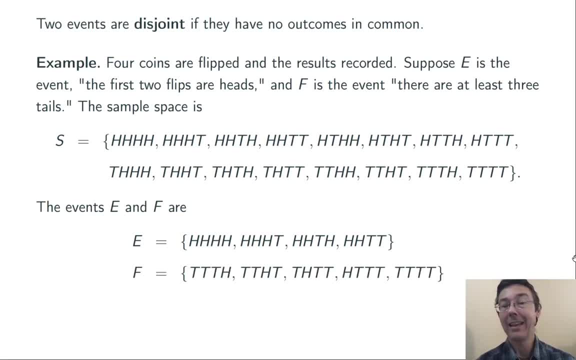 heads, heads, heads and heads, heads, heads, tails and f- at least that there are at least three tails- can be written like this: here we have five outcomes: four where we have three tails and a fifth where we have four tails. notice that there's no overlap between these two sets. there's no outcome that lies. 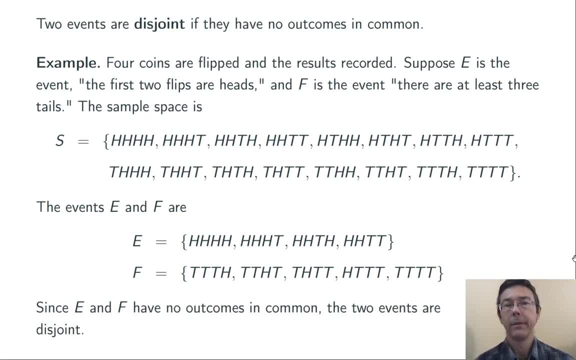 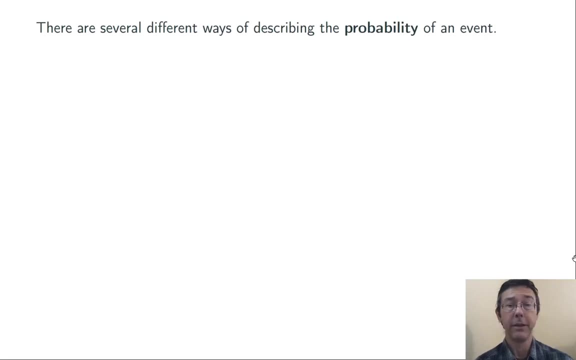 in both of the sets. these are disjoint. to say it in words, it's impossible for both of these events to happen at the same time in one trial of this probability experiment. now, there are actually several different ways of describing the probability of an event, all of which we're. 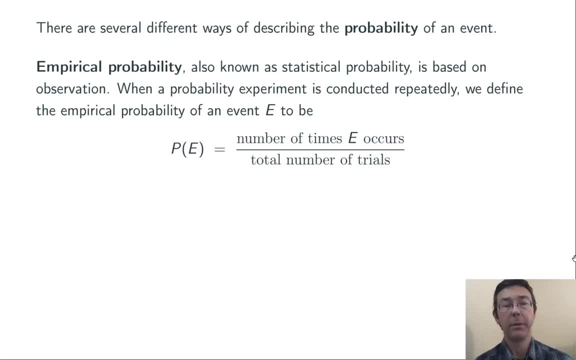 responsible for first is empirical probability or statistical probability, and that's probability just based on observation. basically, we run a probability experiment over and over and over again. we count the number of times that the event occurs and divide by the total number of times we ran the ran, that we ran the probability experiment. this is just going to correspond to the 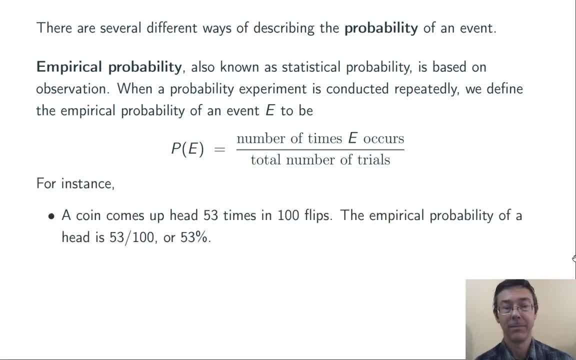 proportion of times the event has occurred in the past. for instance, if we flip a coin a hundred times and it comes up heads 53 times, the empirical probability of the coin coming up heads is 53 and 100 or 53 percent if a poll of seven. now suppose we do a poll of 70 of 750 randomly selected pet. 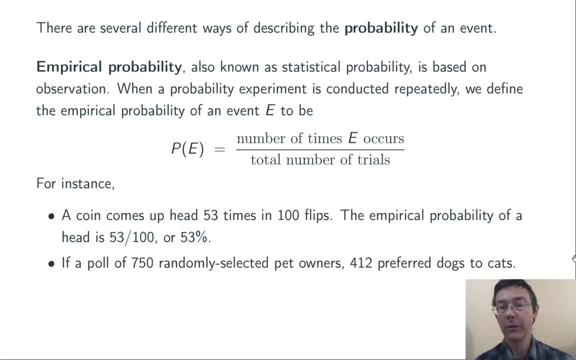 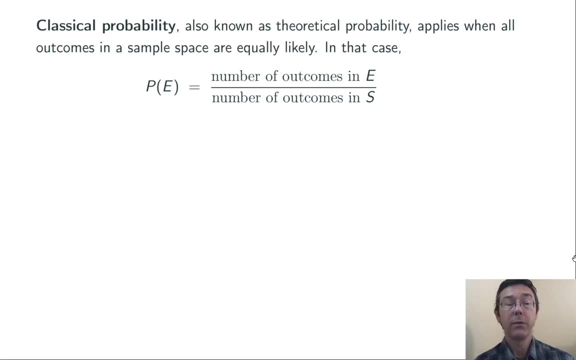 owners, if 412 of them prefer dogs to cats, then the empirical probability that a pet owner prefers dogs to cats is 412 divided by 750, about 54.9 percent. a different way of computing probability is classical probability, also known as theoretical probability, and this only applies when all of the outcomes in the sample space are equally likely. 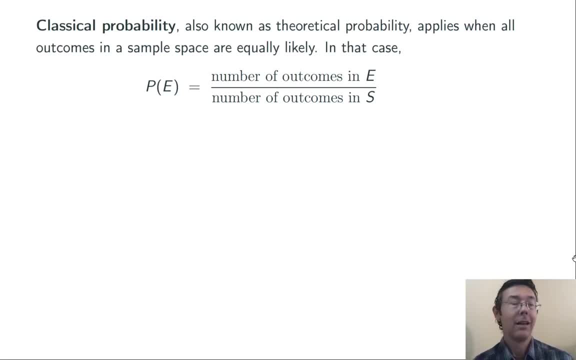 and in that case we count the number of outcomes in the event, count the number of outcomes in the and divide to get the probability. to say this a little more technically, we're doing the cardinality of the set e divided by the cardinality of the set s. so cardinality just means the number of. 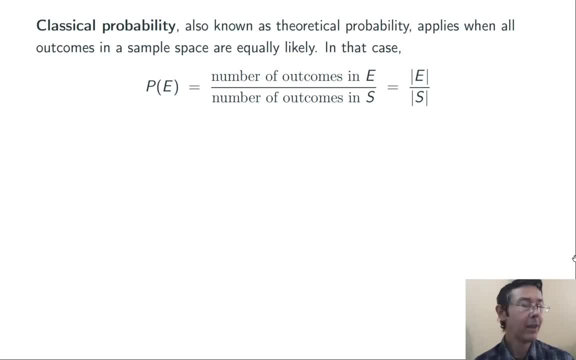 elements in that set. here's the notation sort of absolute value of e divided by absolute value of s, and that just means number of outcomes in each. a couple of examples: roll a fair die. you've got six logical possible outcomes, all equally likely. if we're looking at the simple event, e of 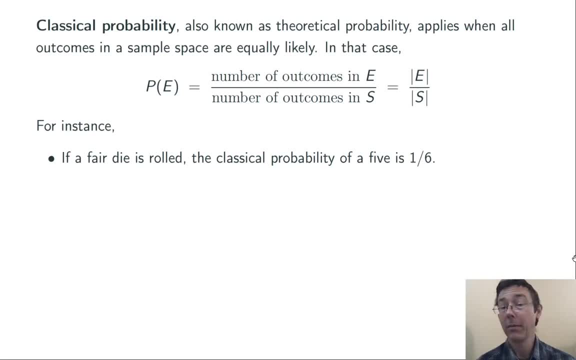 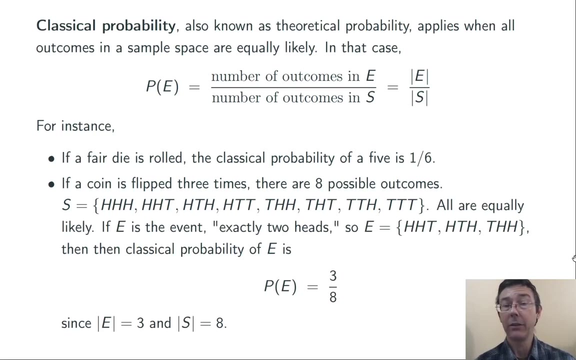 getting a five on that single roll. there's one outcome in that event, so the classical probability is going to be one in six. if we flip a fair coin three times, we have eight possible outcomes listed here, all of them equally likely. let's let e be the event that we get exactly two heads. 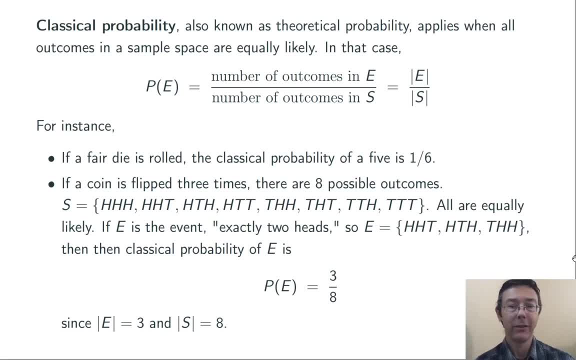 in that event, Heads, heads, tails heads, tails heads and tails heads, heads. So the classical probability of the event E is going to be 3 divided by 8.. There's three equally likely ways of getting exactly two heads out of eight equally likely outcomes possible in total. 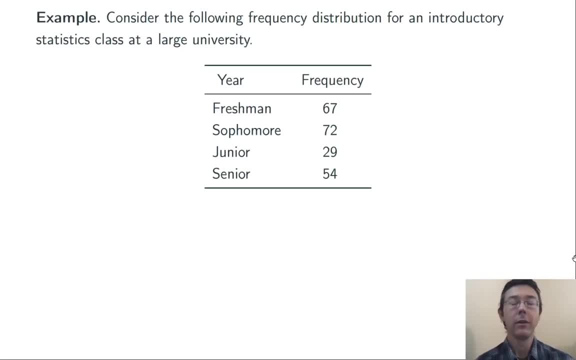 Let's run through an example Here. we have a frequency distribution for an introductory statistics class at a large university: 67 freshmen, 72 sophomores and so on. What's the probability that we randomly select a person from this class and get a sophomore? 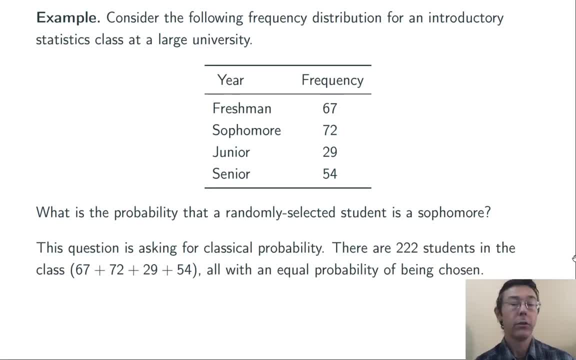 This is a classical probability question. There are 222 outcomes total, 222 students in the class and 72 outcomes that are in the event that we're interested in that. we get a sophomore when we select the person Random. So the probability of randomly selecting a sophomore is 72 divided by 222, about 32.4%. 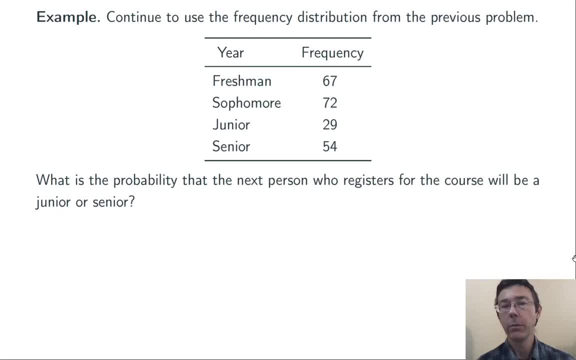 Let's stick with the same frequency distribution and ask a slightly different question: What's the probability that the next person who registers for the course will be either a junior or a senior? This time we're asking for empirical probability. We have data about students that have 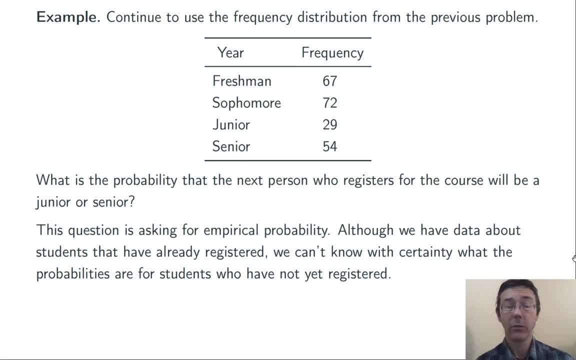 already registered, but we're not sure if they're going to be a junior or a senior. So we're going to calculate the probability of the next person who registers for the course. We're interested in the next person who will register. We can't know with certainty what that probability will be. 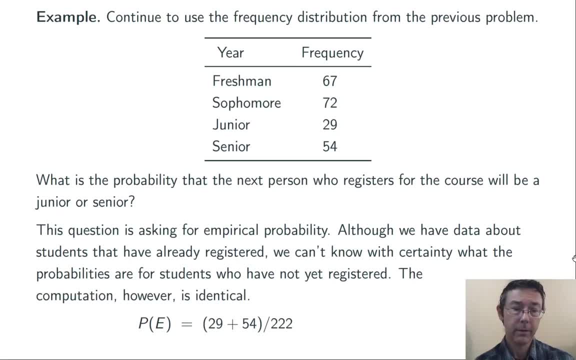 However, the calculation is going to be basically the same. We're going to compute the number of students that have already registered- that are juniors or seniors- so 29 plus 54, and divide by the total number of students that have already registered to get 37.7%. Although the computation 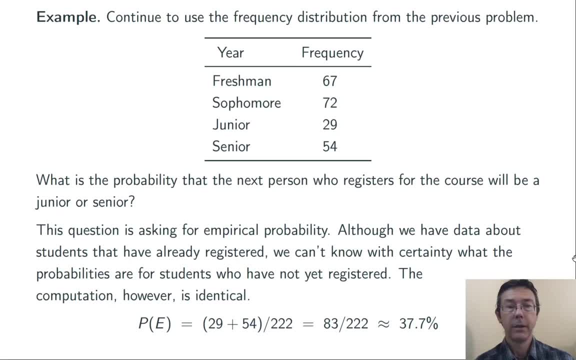 is the same. the philosophy of the problem is that the number of students that have already registered to get 37.7% is the same as the number of students that have already registered to get 37.7%. However, the philosophy behind it is a little different. This time, our probability calculation is based on observation, so it's empirical probability, not classical. 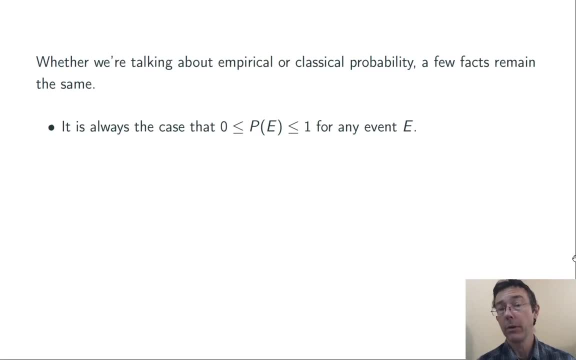 Regardless of whether we're talking about empirical or classical probability, a few facts are always going to be consistent. First of all, for any event, the probability is going to be between 0 and 1.. 0 is going to be an impossible event and 1 is going to be a certain event.